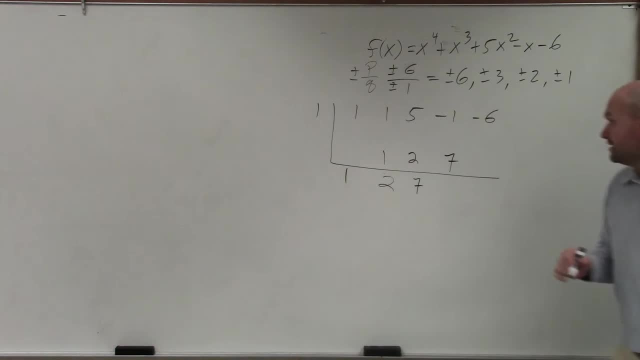 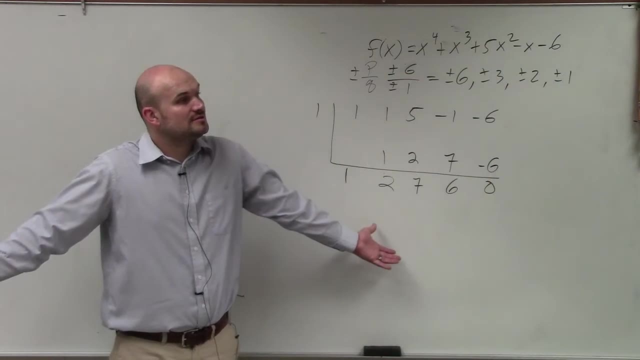 7 times 1 is 7.. Negative: 1 plus 7 is going to be 6.. 6 times 1 is negative 6.. 0.. 6 times 1 is not negative 6.. Let's say it works though. 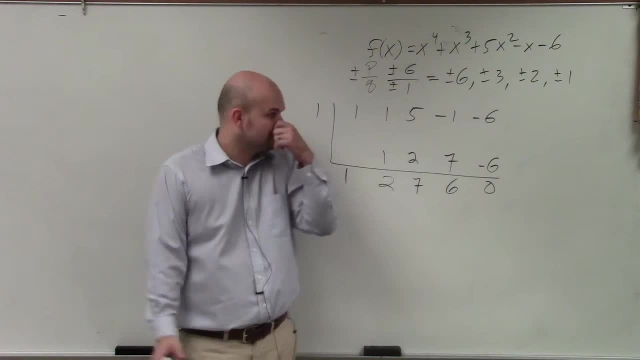 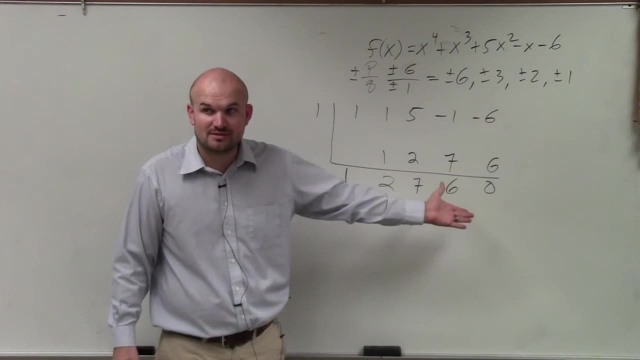 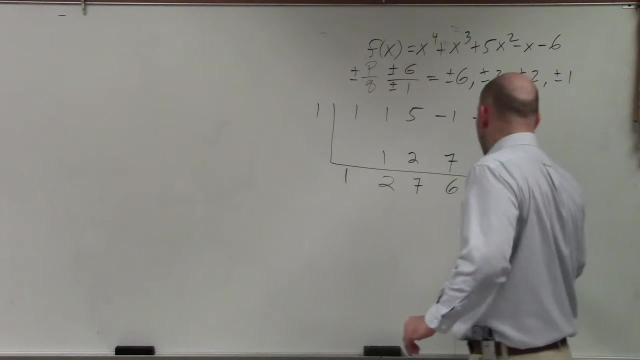 Yeah, but it works. Wait, negative 6 is negative 6.. Sorry, sorry, sorry, But does everybody believe that this works? OK, now good. However, ladies and gentlemen, as I mentioned, this is: this is a quadratic constant. 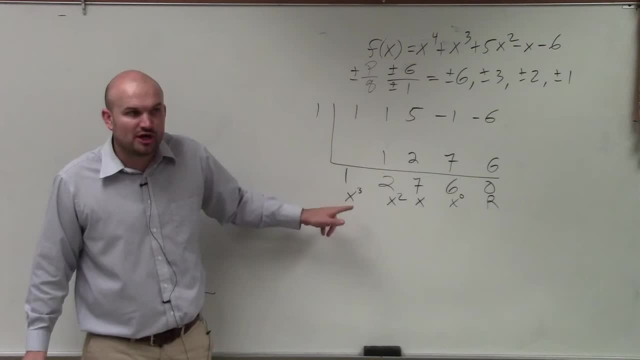 That's a cubic polynomial right It's x to the third. It's a cubic. You're not going to be able to factor this. I mean, you might be able to look at it. I'm not going to be able to factor this. 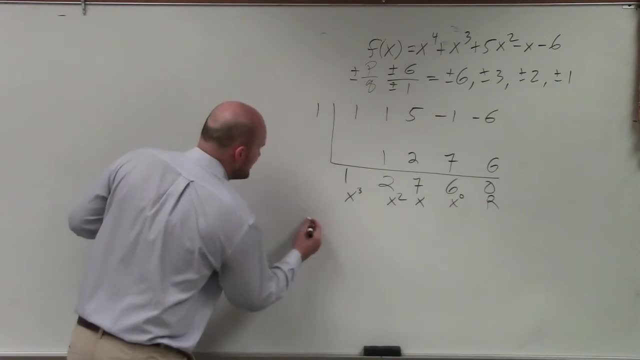 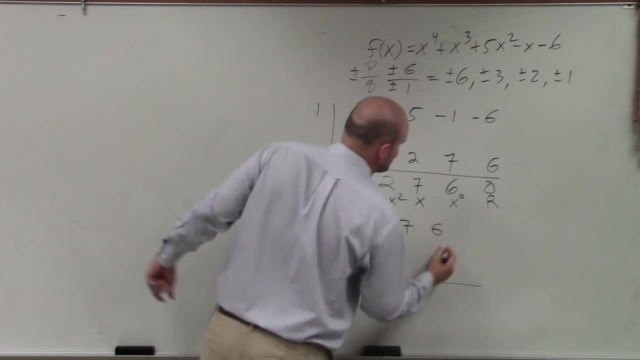 So I know So. therefore, I need to further refine it, right? So let's go out and try negative 1, and see if also negative 1 is a factor. So I'll bring down the answers: 2,, 7,, 6, and 0 is the remainder. 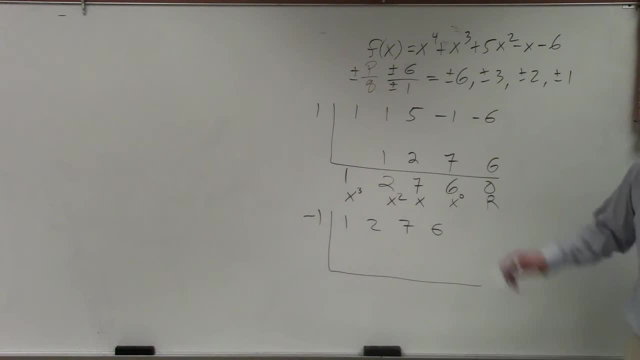 So I'm not going to worry about that. Yes, Does this mean you only have three 0's or four 0's, Four 0's? OK, So let's go and try negative 1.. See if negative 1 works. 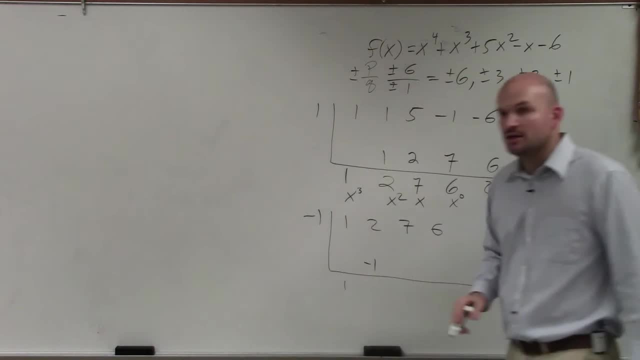 I bring down the: 1. 1 times negative: 1 is Negative. 1. 2 plus negative: 1 is 1.. 1 times negative: 1 is Negative. 1. 7 plus negative: 1? Negative: 6.. 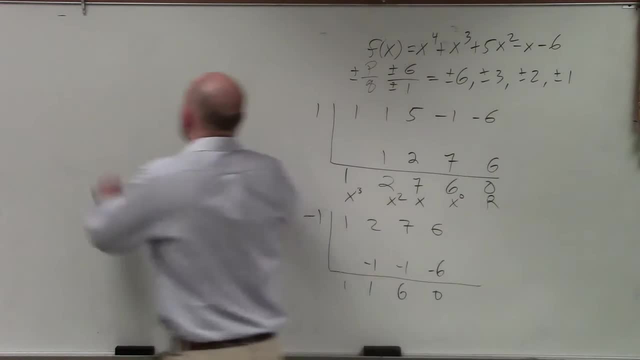 And that works too. So right now my factored form: if 1 is a 0, what's my factor? x minus 1.. If x minus 1 is a 0? x plus 1.. x plus 1.. 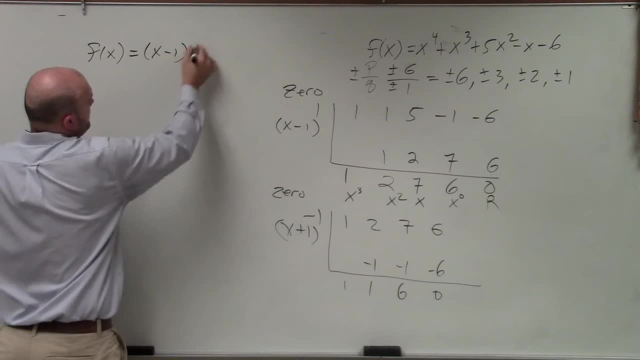 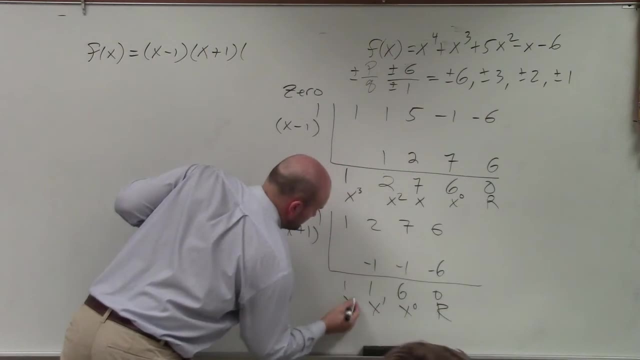 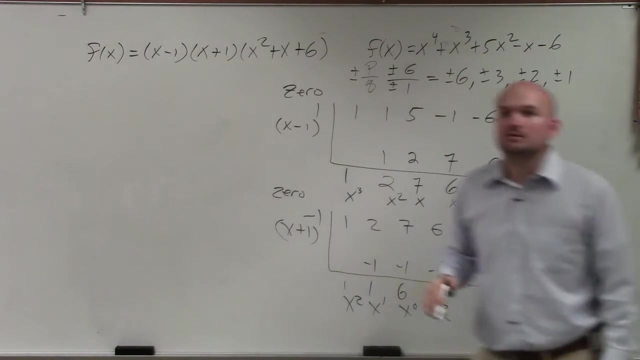 So Sam is canceled for today. The what Sam is canceled for today. He will be next Thursday, That's OK. That's OK. I'm looking down. Oh really, Shh, Listen, Listen. Does everybody agree? that's my factored form. 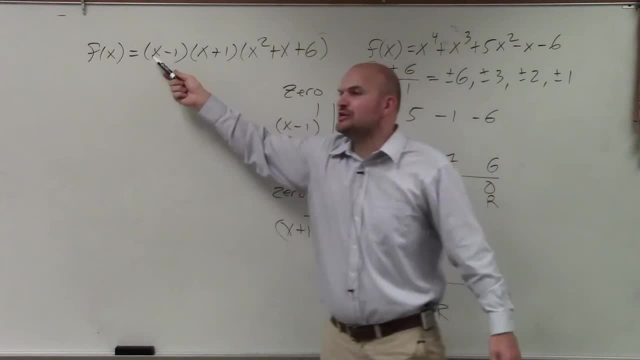 Yes, Yes. Now if you were to do a 0 product property, we already know that's a 0, 1.. We already know that's a 0, negative 1.. However, this one, we have to factor it. 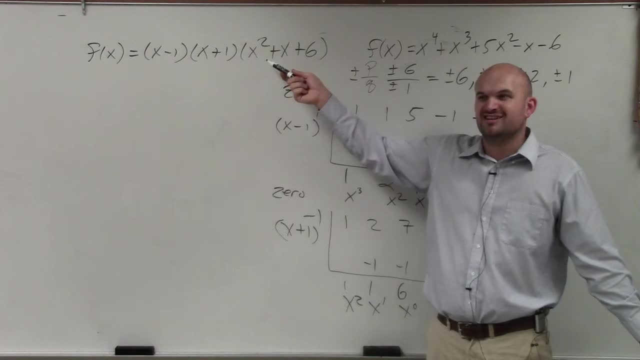 But look at that. What two numbers multiply to give you 6, add to give you 1? None, None, Crap, It's not factable. It's not factable. So guess what you have to do? Quadratic formulas. 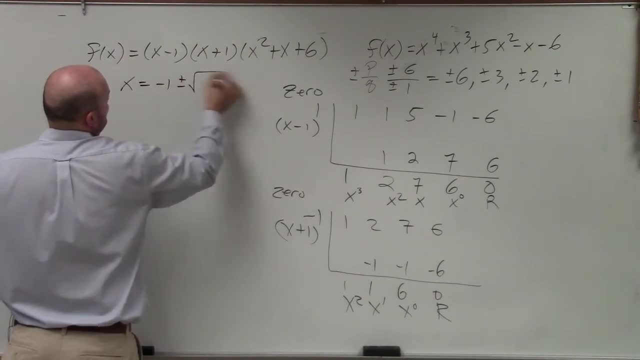 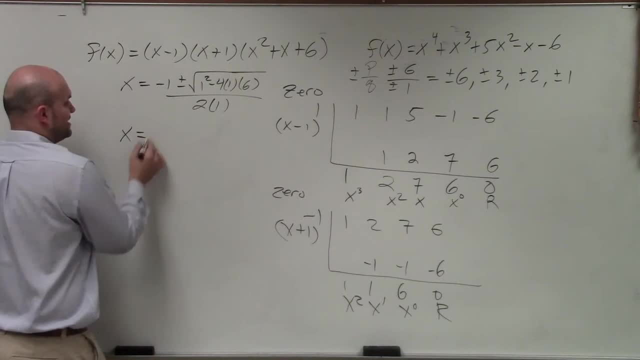 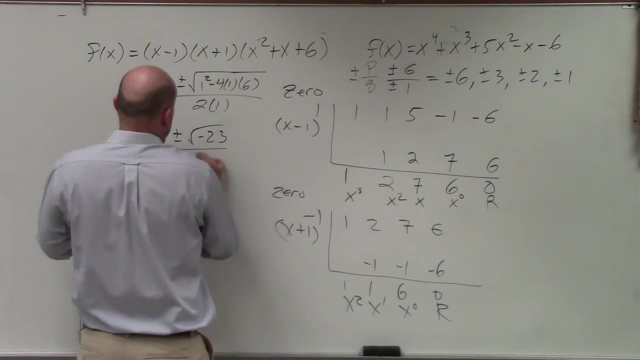 Oh, Oh, Oh, Oh, Oh Oh. I got to tell you guys something. one last quick thing. So that's 1 squared, That's the square root of negative 23 over 2.. Shh, So I could also write that as x equals negative 1 half. 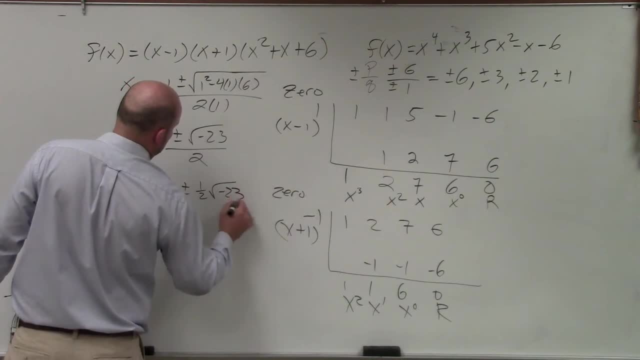 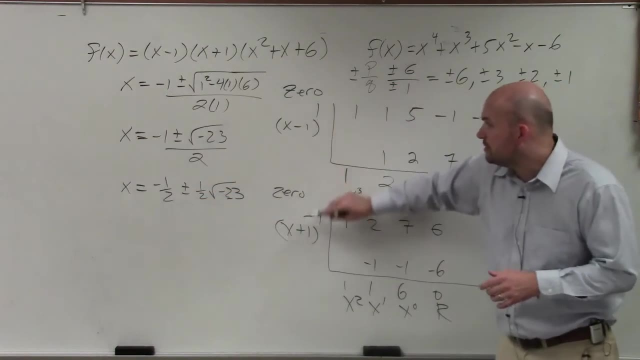 plus or minus 1 half times the square root of negative 23.. So what I want you guys to understand here is: there's two complex solutions, right, And there's two real zeros, right. What I want you guys to understand is write down: 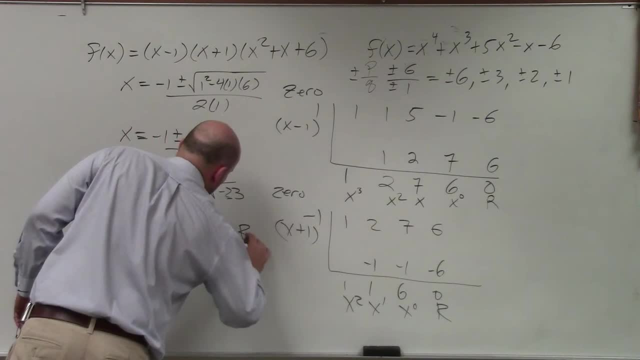 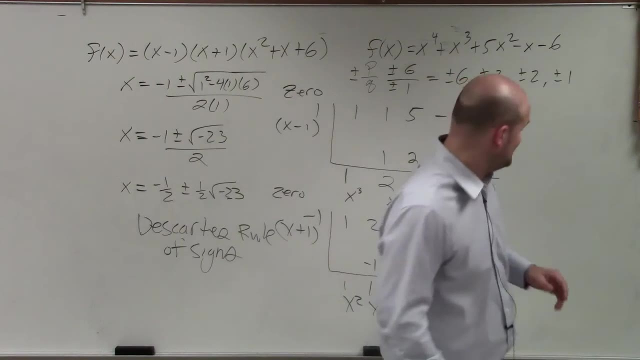 Descartes' rule of sines. Write it down, because you're going to need to probably go and look it up there. I have videos online, but I want you guys to see what we're talking about. What Descartes' rule of sines? you guys need to see this. 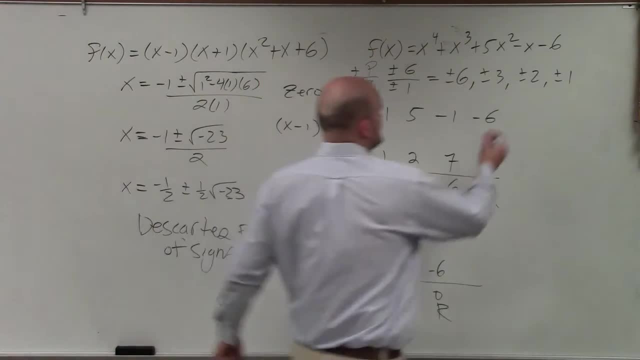 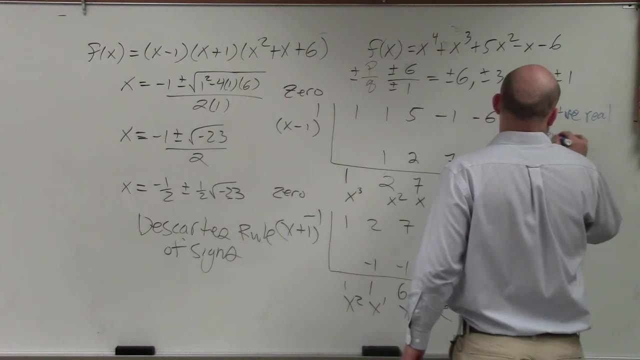 and visualize this. What Descartes' rule of sines says is: the number of positive real zeros is equal to the sine changes of your polynomial. Well, how many sine changes do I have? Just one. So what they're saying is there's only one real positive. 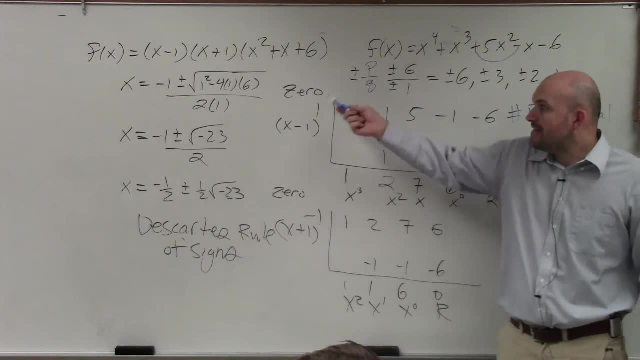 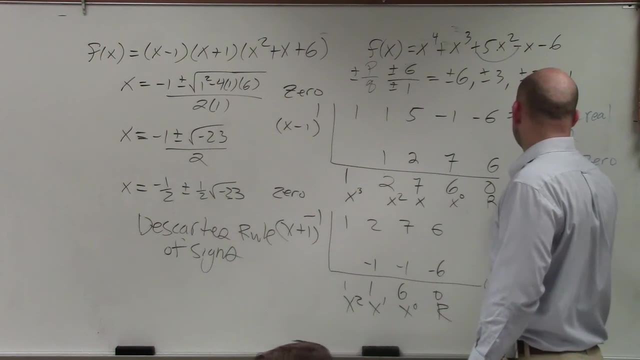 zero. And is that true in my example? Yeah, there's only one real positive zero, right. And then the number of negative is the number of negative is the number of sine changes. I don't have to go through it, Just remind me to review this again. 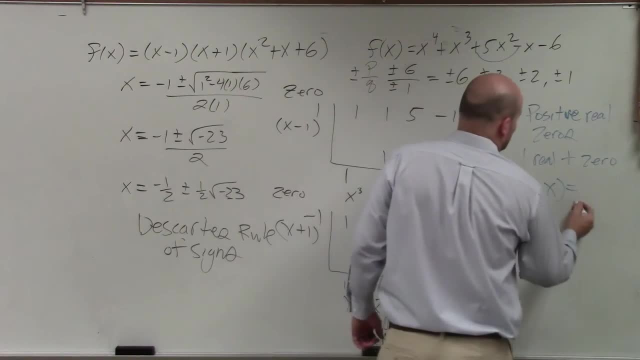 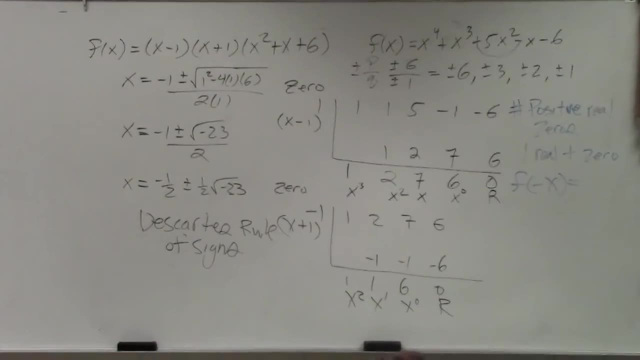 But it's the number of sine changes of f, of negative x, And then the number of negative zeros is equal to the number of negative zeros. I'll go back over that. I do have homework, I do have videos on it, So please plan to get your.